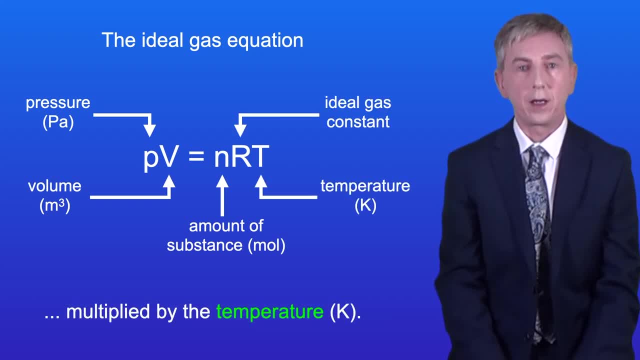 by the ideal gas constant multiplied by the temperature in Kelvin. Now it's really important that you learn this equation and you need to learn the units. In my experience, if a student makes a mistake with this equation, it's often because they got the units wrong. So in this video we're going 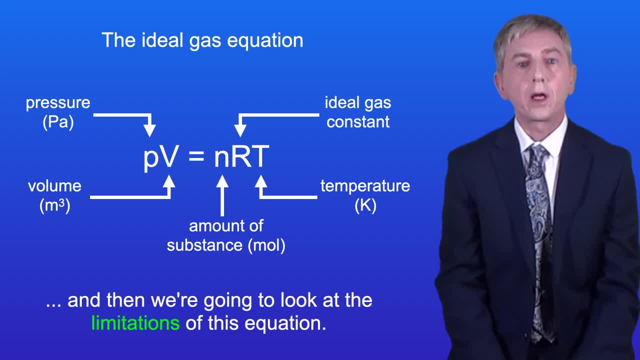 to take a closer look at the ideal gas equation, and I'm showing you that here: Pressure in pascals multiplied by volume in meters cubed equals the amount of substance in moles multiplied by the equation and the units. And then we're going to look at the limitations of this equation. Okay, 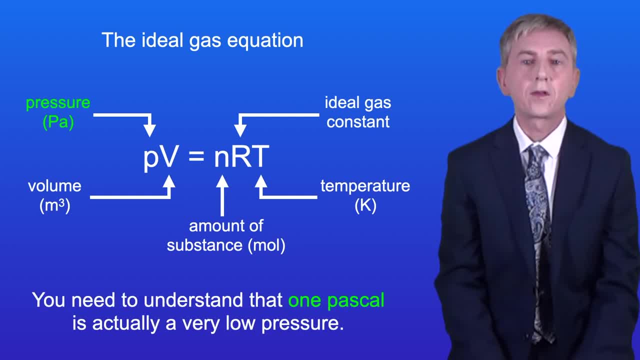 the pressure of the gas has to be in pascals. Now you need to understand that one pascal is actually a very low pressure, so usually gas pressure is given in kilopascals. To convert from kilopascals to pascals you need to multiply by 1000.. The volume of the gas has to be in meters. 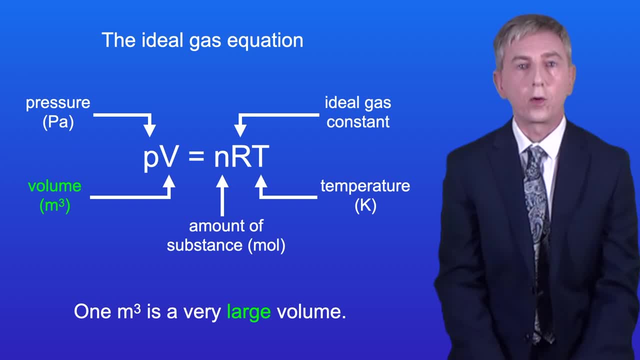 cubed. Now, one meter cubed is a very large volume, so in chemistry gas volumes are usually given in either decimetres cubed or centimetres cubed, So you need to remember to convert the gas volume to meters cubed, and this is the one thing that students 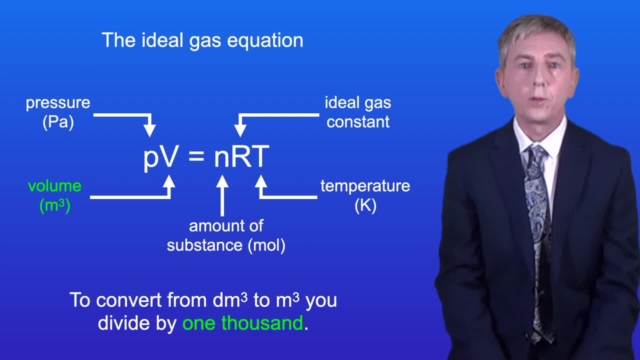 often forget. To convert from decimetres cubed to meters cubed, you divide by 1000.. And to convert from centimetres cubed to meters cubed, you divide by 1 million. Coming up, we'll continue looking at the ideal gas equation and I'll discuss the assumptions we make when we're using the equation. 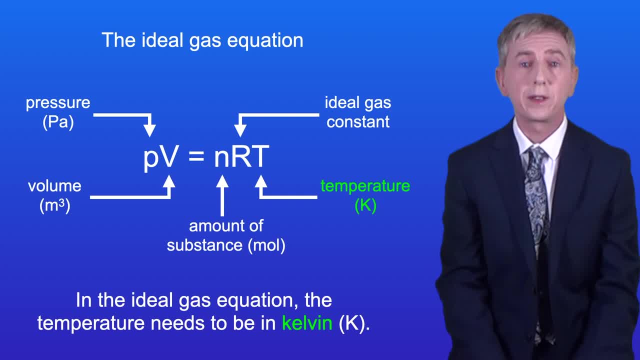 Okay now, in the ideal gas equation, the temperature needs to be in Kelvin, and this is a unit that you might not have seen before. You'll notice that we say Kelvin, not degrees Kelvin. To convert from degrees Celsius to Kelvin, you need to add 273.. And to convert from Kelvin to degrees Celsius, you. 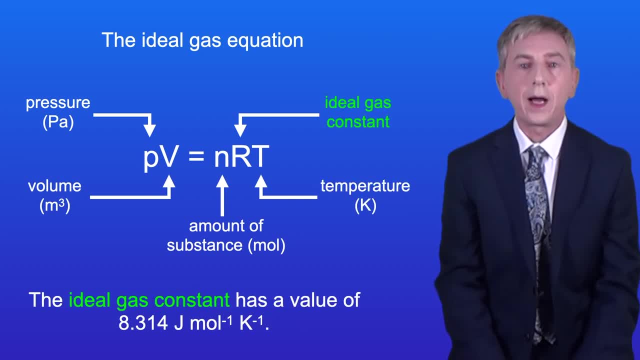 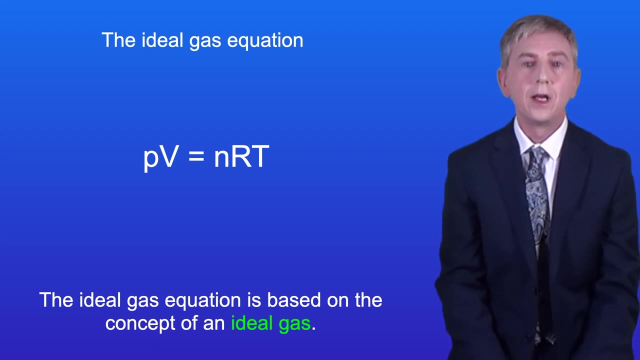 need to subtract 273.. The ideal gas constant has a value of 8.314 joules per mole per Kelvin, And I that you're given this in the exam. Okay now, the ideal gas equation is based on the concept of an ideal gas, and for an ideal gas we make the 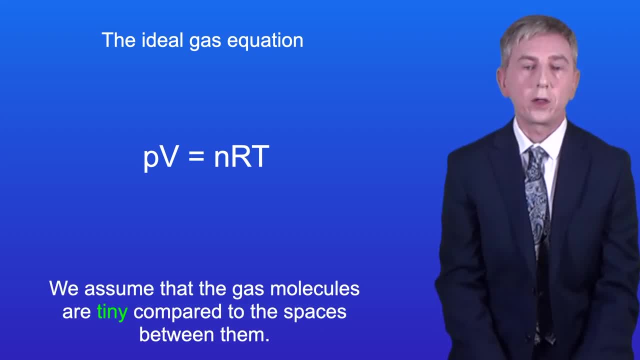 following assumptions: We assume that the gas molecules are tiny compared to the spaces between them. We also assume that there are no forces acting between the gas molecules. We assume that the gas molecules move randomly And, lastly, we assume that when the gas